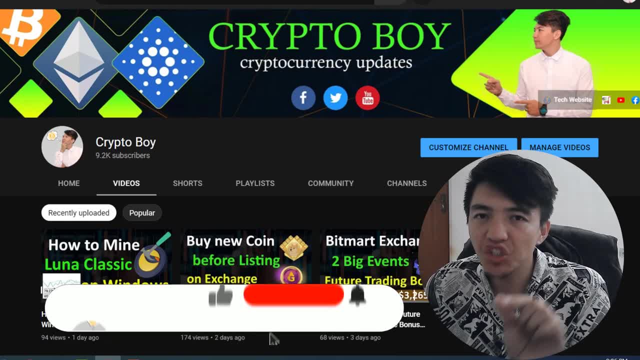 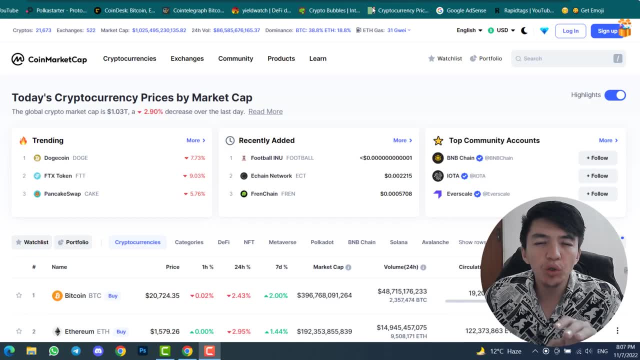 meme points, even about indicators or trading strategy. so make sure, click on the subscribe button, hit the bell icon to get notification while upload any video. so, as i told you, in this crypto market we have 21 673 cryptos like a coins, but how to find the coins that are ready? 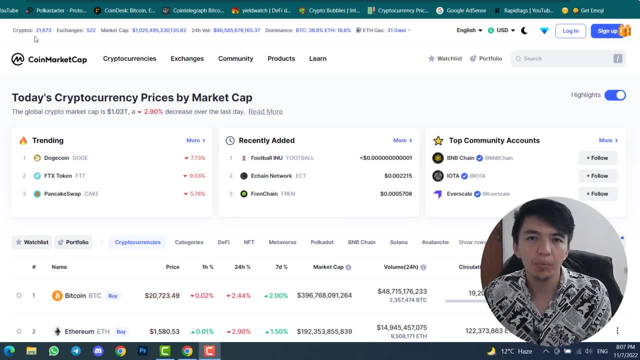 for pump, how to find any coins while pumping, because searching the coins, doing your technical analysis using indicators, it will take lots of time, but there are a short period of time, or i can say there are a short time like shortcut time. you can easily find any coin before pumping. i will show you inside this video. so this is the 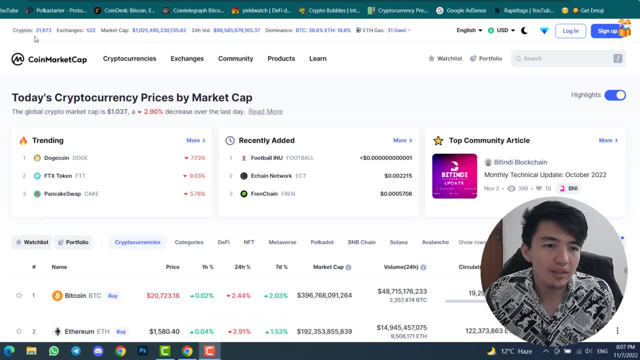 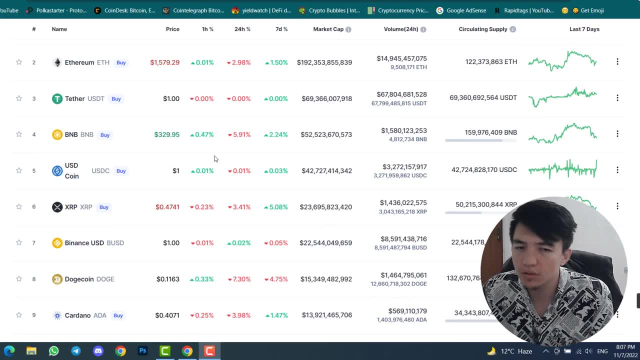 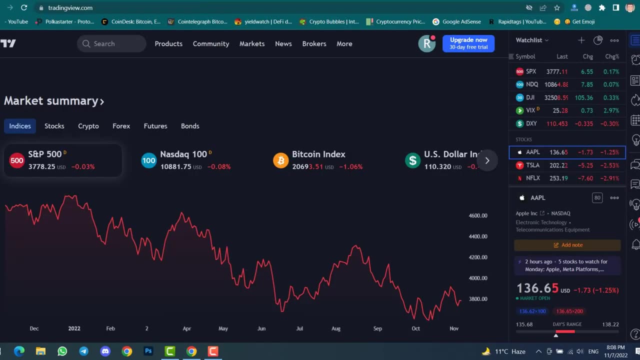 best platform. everyone can use it. so you can see, this is coinmarketcapcom. inside coinmarketcap you can find the whole cryptocurrencies, the whole meme coins, the tokens. but this is the tradingviewcom. inside tradingviewcom, we can use our trading strategy so that everyone can make profit, so that everyone can find any cryptocurrency before they pump. 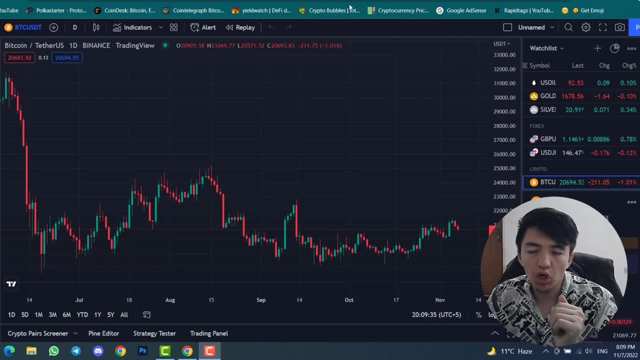 so this is tradingviewcom and you can see this is the chart. so if you know about a trading view, crypto skinners, so you must know about this trading strategy. you must know how to find any cryptocurrency before they pump, Because inside this video we will use crypto screeners and I will show you what filter you should use in order to find any cryptocurrency before they pump or in order to find any cryptocurrency while pumping so that you should make a profit quickly. 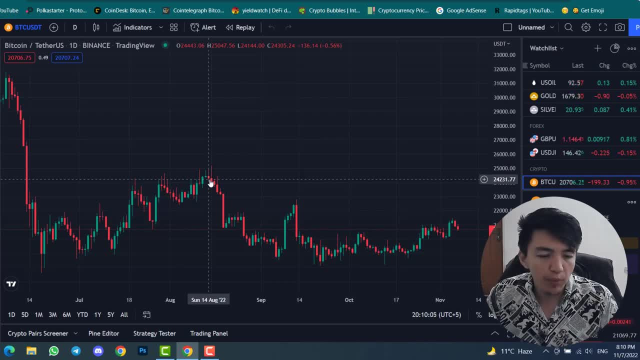 So once you come on tradingviewcom, so simply click on crypto pairs scanner or you can click inside this arrow button Once you click in here, so you will see three options: stock screener, forex screener, crypto pairs screener. 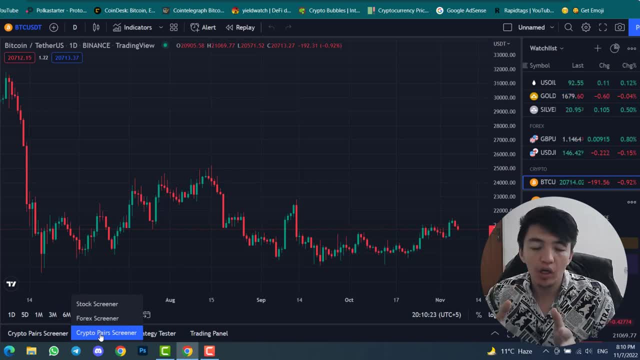 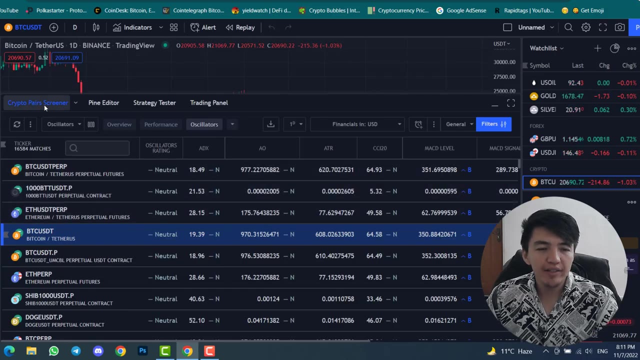 So you can find any coin, any forex coin or, I can say, any stock coin, before pumping not only cryptocurrency, but you can use forex and stock also with this trading strategy. So simply click on crypto pairs screener and then you can see. this is the crypto pairs screener. 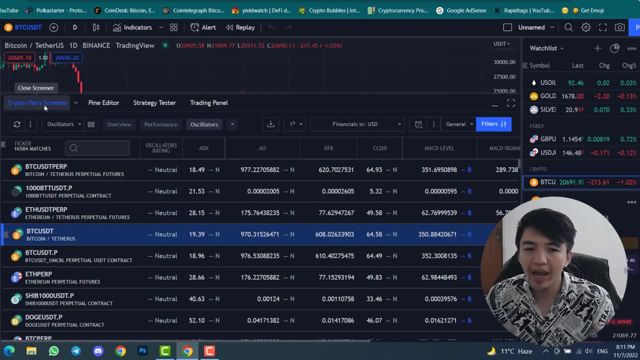 So in here you don't need to do anything, You don't need to change The only thing that I will show you inside this video. make sure to make that changes So once you come here. so simply click on filters, don't change anything. click on filters. 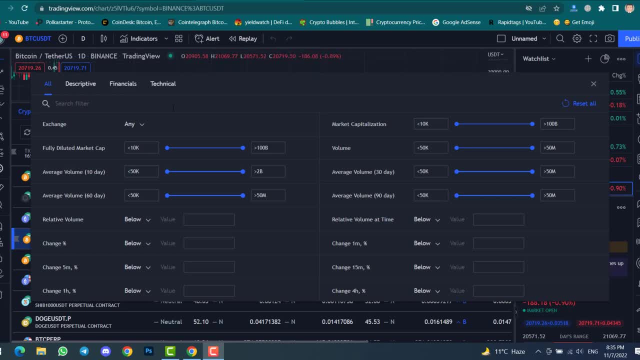 So, once you come here, first of all we need to select our exchange. So simply click on any option Now, select Binance, and then I will select Bitgate, so you can select any exchange that you want. Okay, and the next option is. the next option is simply to search. 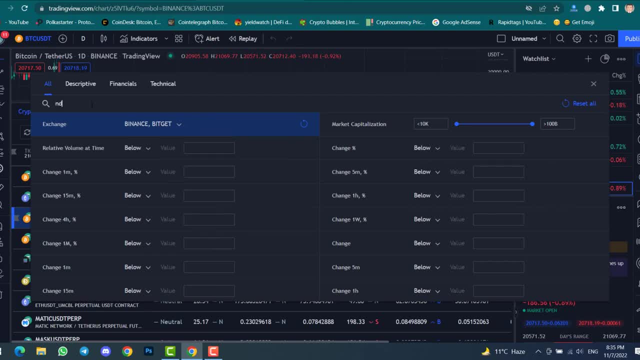 So let's search about NDI indicator: NDI. So once you type NDI, it means that positive directional indicator, negative directional indicator. So we just want to active negative directional indicator. for that, Click on below. So now select crosses down. 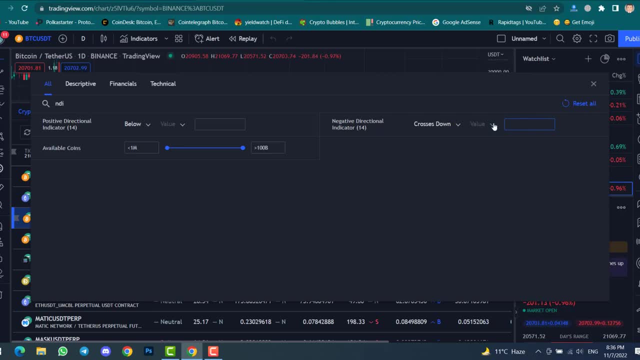 For the value, select positive directional indicator. So it means that whenever Negative directional indicator crosses down positive directional indicator, it means that the coin is just pumping, the coin is ready to pump. This is how you can find any coin before they pump. using negative directional indicator crosses down positive directional indicator. 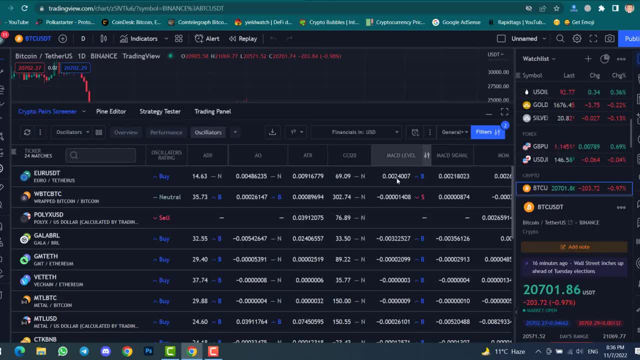 Now simply click on cross button So you can see in here: this is all the coin that are ready for pumping. These are all the coin like before they pump. So in here I will type USDT only. I just want to find the coin with the USDT pair. 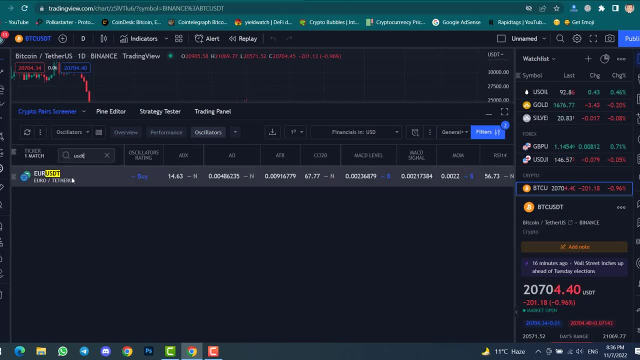 So you can see, only I have one coin. only I have one coin- EUR with USDT. This is ready to pump, But for that make sure to select the time frame. So with this trading strategy, 4 hours will work the best. 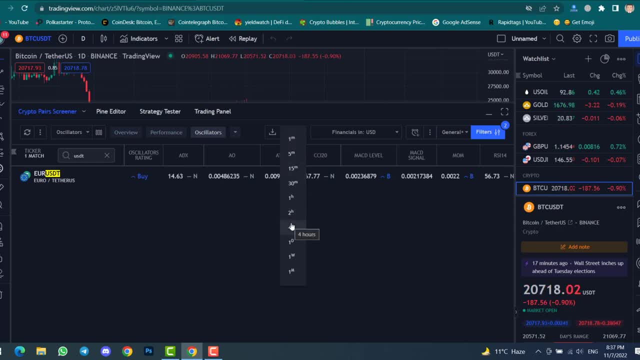 So with this trading strategy, 4 hours will work the best. So with this trading strategy, 4 hours will work the best. So for now, I'm just using the free version of tradingviewcom. So for now, I'm just using the free version of tradingviewcom. 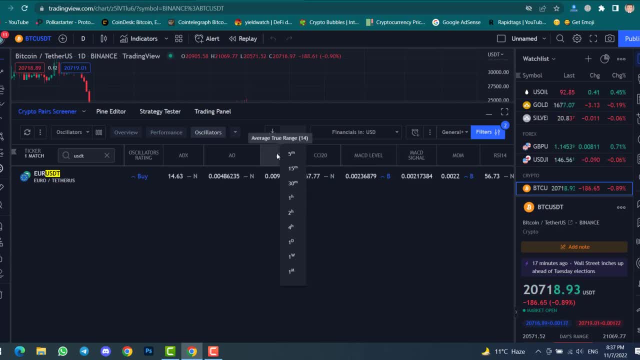 If you want to use the lower time frame, you need to just pet the tradingviewcom. If you want to use the lower time frame, you need to just pet the tradingviewcom. If you want to use the lower time frame, you need to just pet the tradingviewcom. 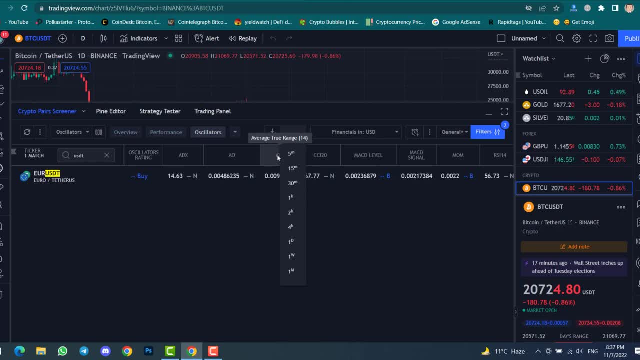 Just buy the premium version. So for free version you can only use the higher time frame, like one day, one week, one month. Just buy the premium version. So for free version you can only use the higher time frame, like one day, one week, one month. 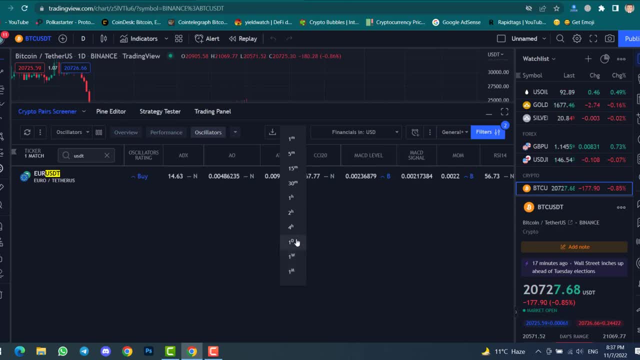 So for free version you can only use the higher time frame, like one day, one week, one month, But for now I will select one day, because this is a free version of tradingviewcom. And then about oscillator rating: simply click on it and then click on any option. 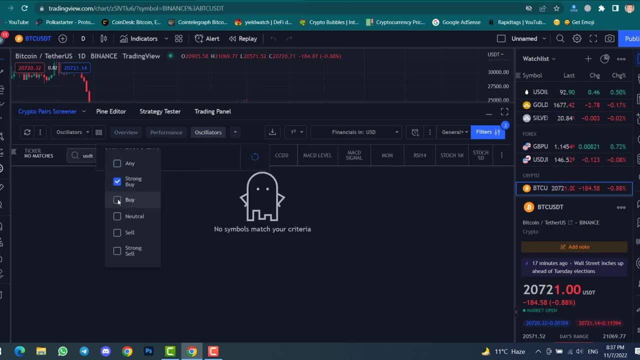 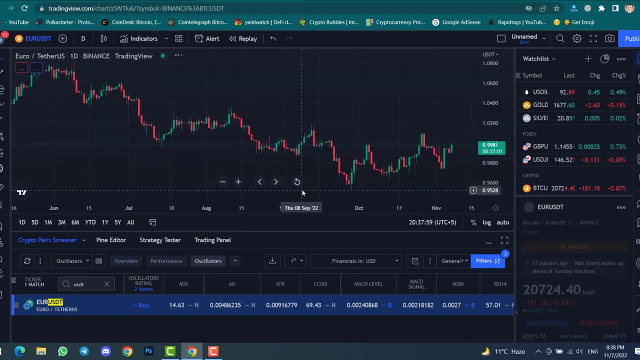 In here. I will select a strong buy and then I will select buy option. So for now, you can see we have only one coin which is ready to pump. Simply click on this Now we will check the chart whether the price is ready for pump or not. 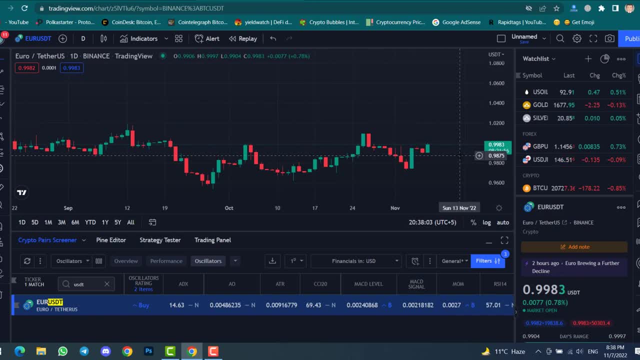 So yes, you can see, in here It means that the price is just ready to pump, or the price is now just pumping. And here you can see, we have somehow, I can say in here bullish engulfing, And then I can say this: one bullish harami. 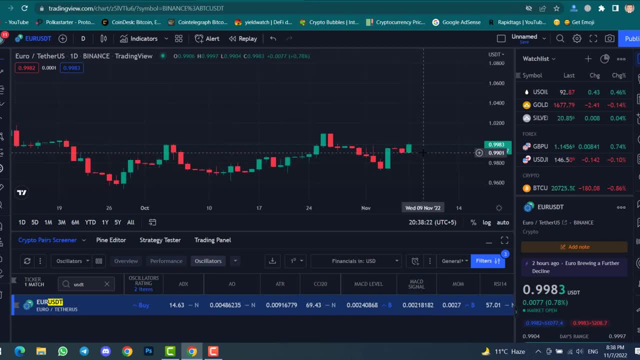 No, I cannot say it. I cannot say it. So it means that now this coin, the price is ready to pump, Or we just found a coin before they pump. You can see, But for now, unfortunately, for daily time frame, we have only one coin. 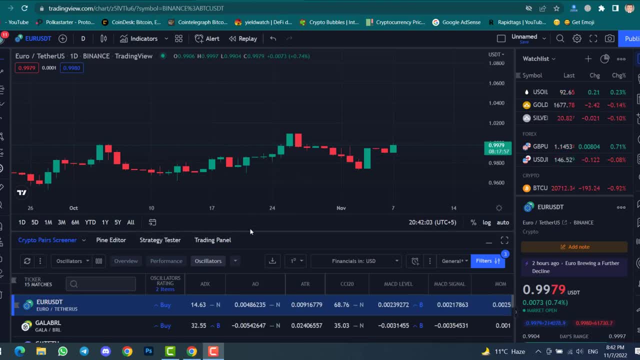 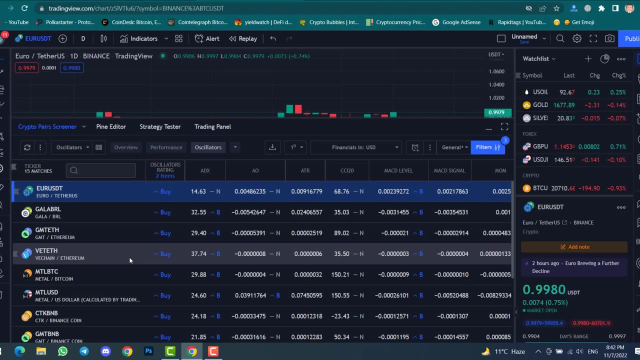 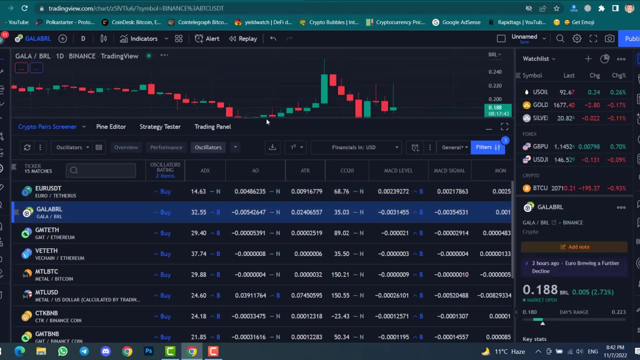 Okay, now if I remove USDT from here, So you can see, we can check the all coins with any pairs, like Ethereum pair, BTC pair, USDT pair, BNB pair. So if I show you Gala with B or L, So let's see whether this coin is ready for pump or not. 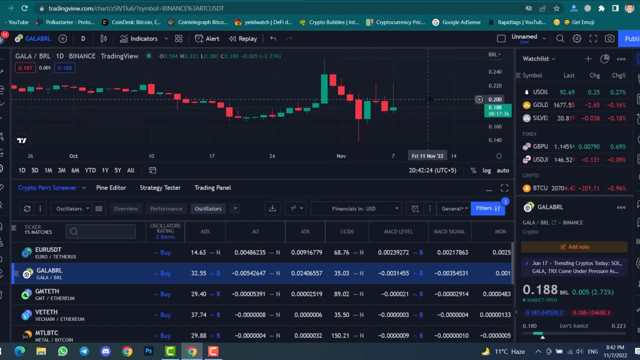 Then you can see: yes, the coin is ready for pump Because we have about hanging man in here. And then you can see: So if you check other coin, GMT with Ethereum pair, So in here again, you can see the coin is ready for pump. 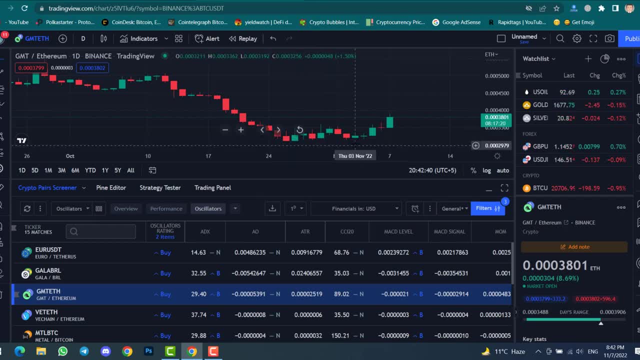 Like in here, we have bullish engulfing. Or then you can see: yeah, the coin is just pumping, or the coin is ready to pump. Or if you check with Ethereum again, you can see the coin is just pumping or the coin is. 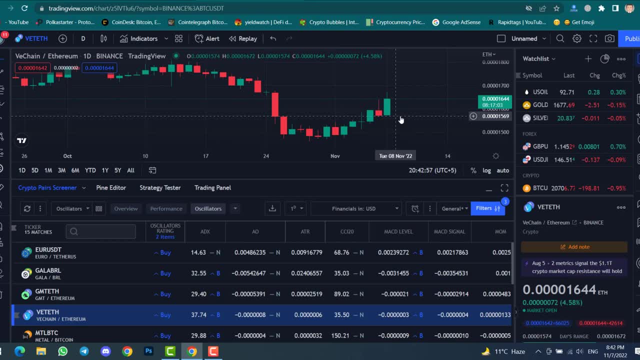 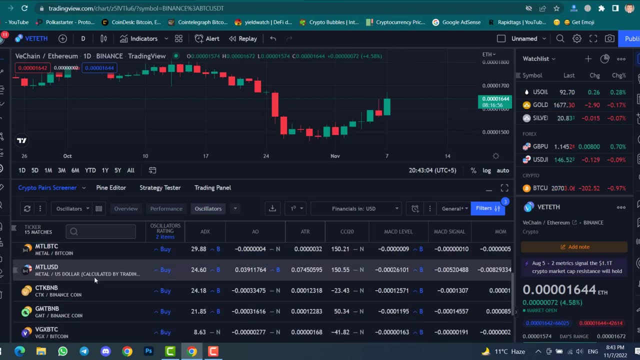 Ready to pump. This is how you can find any coin before they pump. This is how you can find any coin while pumping. So I hope you understand this video. If you check one by one, like you can see MTL with USDT. 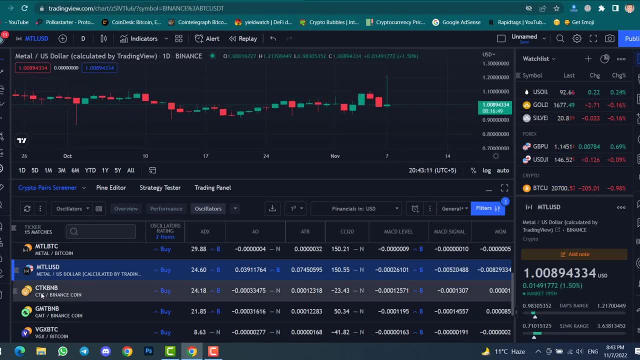 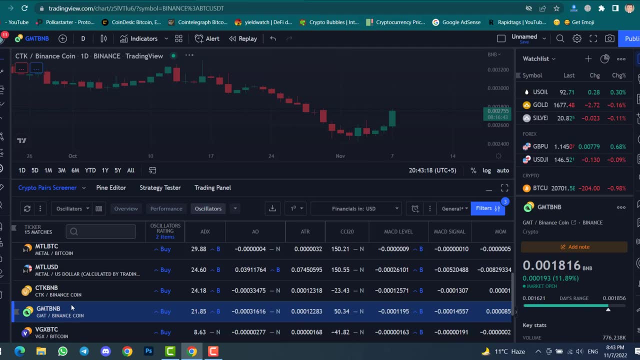 Yeah, you can see. And then if I show you CTK with BNB, So the coin is just ready for pumping, And then if I show you GMT with BNB, Also, the coin is ready for pump. VGX, VGX. 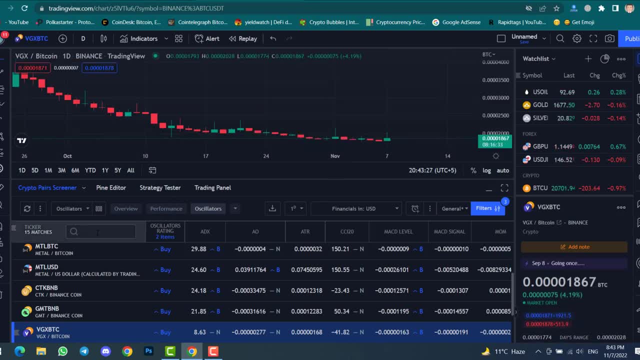 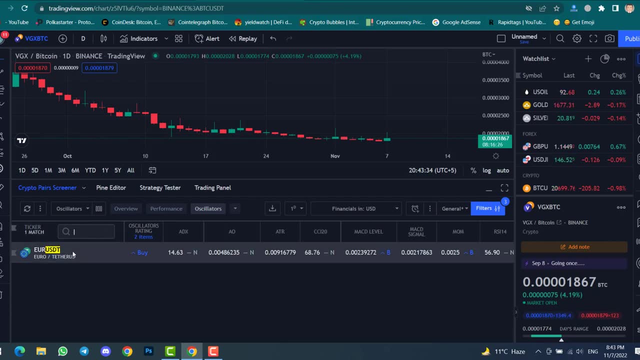 VGX with BTC. So it means that in here if I show you the USDT pair, So for USDT pair only one coin is available. But if I remove USDT, so you can see there are about 50 matches. 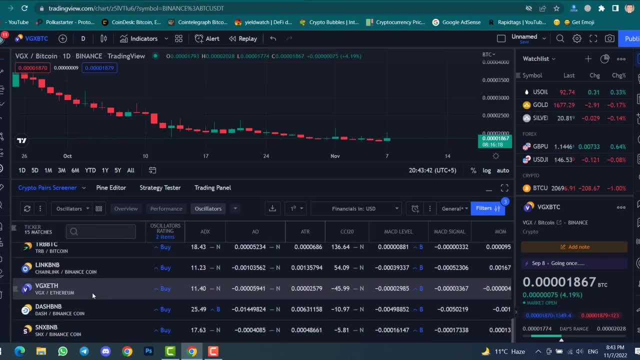 You can see in here 50 matches. So this is all the coin that are ready for pump. You can see the buy signal Oscillator. threading is buy signal. You can see Buy signal. buy signal. It means that this is the time. 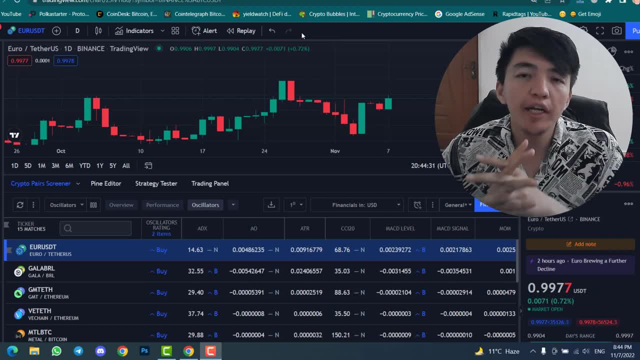 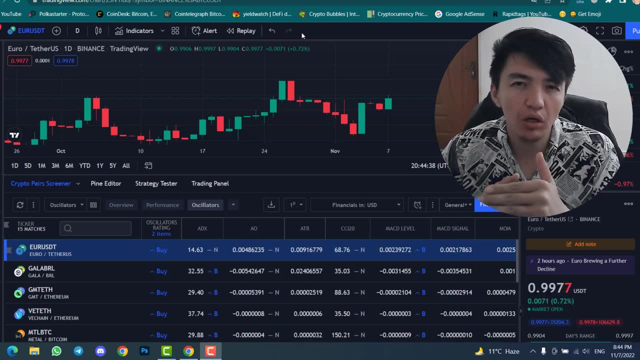 To buy this coin. So this is the best way to find any coin before they pump Or to find any cryptocurrency while pumping. So if you have the paid version of tradingviewcom, So I recommend you to use 4-hour time frame.